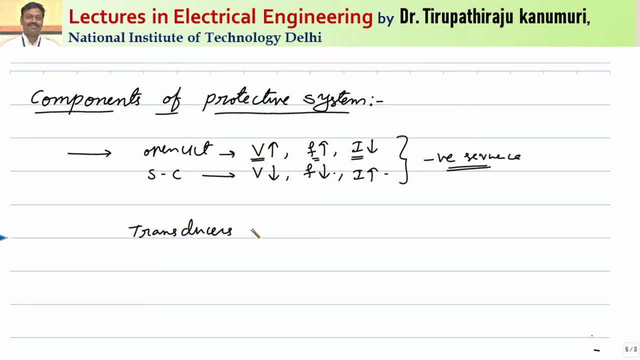 sense the fault. So for that we need the transducers. So this transducers can be either current transformer or a voltage transformer. So this current transformer or the voltage transformer, these are used for decreasing the value of the voltages or the currents Generally, irrespective of the primary current, because we know in our power system the current can be very high. 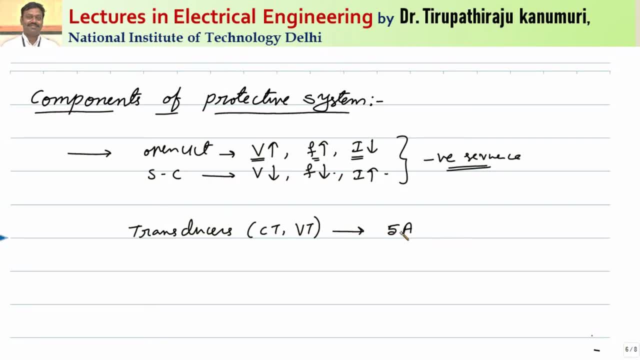 It may reach up to thousands of amperes. But if that much current cannot be passed through your relay because it is not safe for the personnel who are operating and that much magnitude cannot be measured by your relay, So it is generally stepped down to a 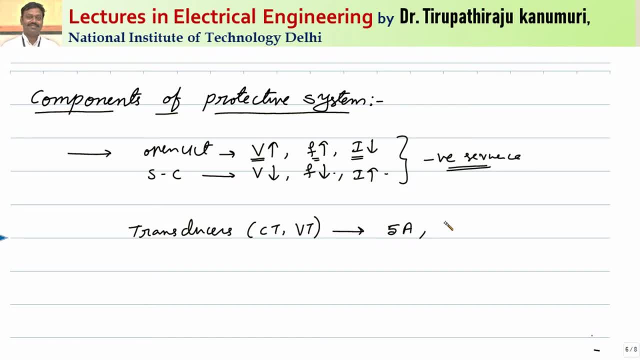 standard value of 5 amperes, and similarly, the voltage will be stepped down to a value of 110 volts so that it can be easily measured. So this is the basic purpose of the transducers. So once the transducers are there, After that we need a relay to detect what particular parameter you want to measure. 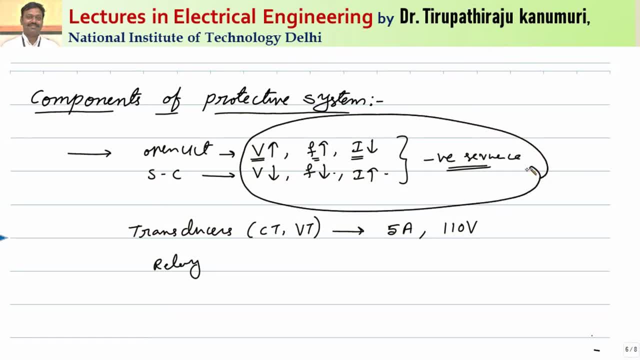 That means. so, out of these different parameters, whatever you want to measure, So this will be done by the relays. So after relays comes the, because the relay is there. So this relay is going to operate your circuit breaker. Generally, the relay cannot operate the circuit. 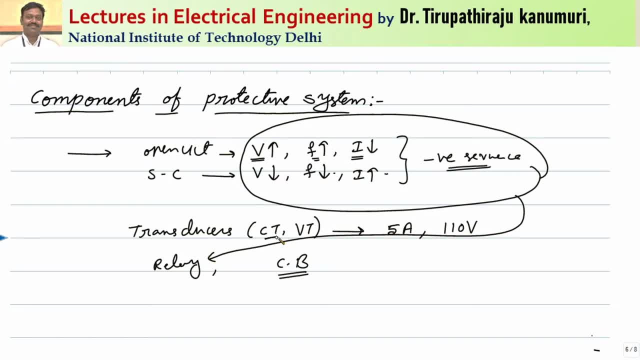 breaker directly, because the burden on this transducers CT and VT should be, or potential transformer should be, as minimal as possible If these circuit breaker operating circuits is completely directly connected to the CT or PT, so that much power should be supplied from your transmission line. So whenever that much power is, 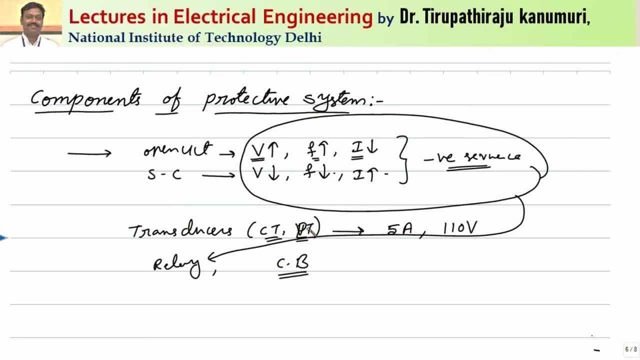 supplied by your transmission line that are going to affect the characteristic of your system. You have seen this in the case of measurements, That is, voltmeter, ammeter method, you have seen there. So there, you have seen that, if you want to measure, 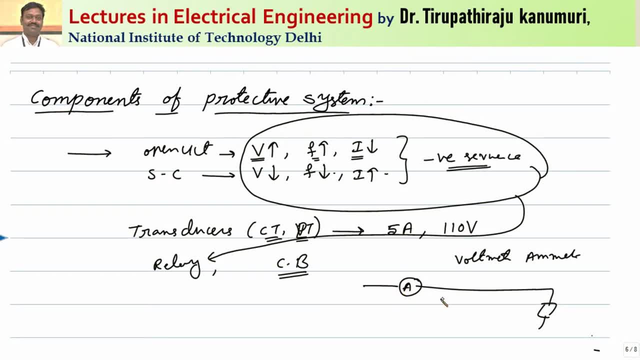 there is some load. If you want to measure the characteristics takes you can. you will connect an ammeter and a voltmeter to measure this value of the resistance. let us assume i want to measure this resistance. what we do? we take the ratio of voltage divided. 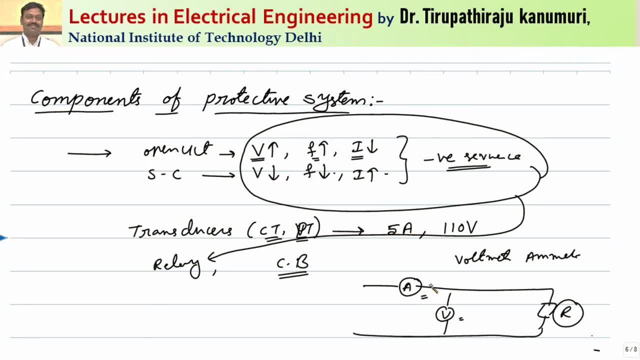 by current. so when you want to measure it here, what happens? this ammeter is going to carry the current that is required for the voltmeter. also, this is my load current and this is my shunt current, or the current passing through the voltmeter. this entire current passes through. 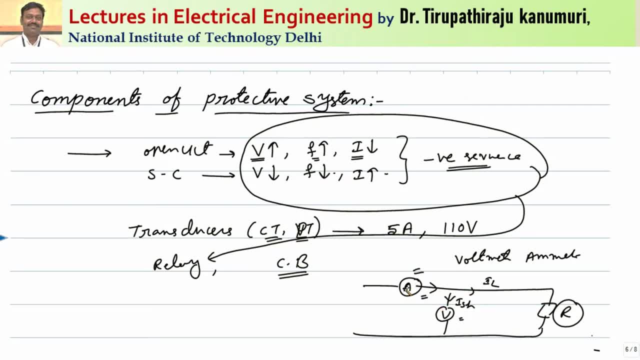 this, so it gives the error. similarly, if voltmeter is kept first, then ammeter is kept. that is also going to affect so what i want. the value of the current taken by the voltmeter or the amount of the power consumed by the ammeter should be as minimal as possible so that the errors will be. 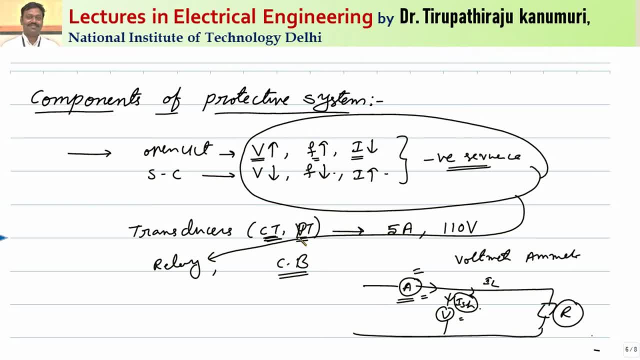 minimum. so same thing is the case here. the ct and pt should not load your system. that's why a separate circuit will be used for operating those things. so that circuit is called as the trip circuit. so the trip circuit will take the power from a separate source, so that burden will not. 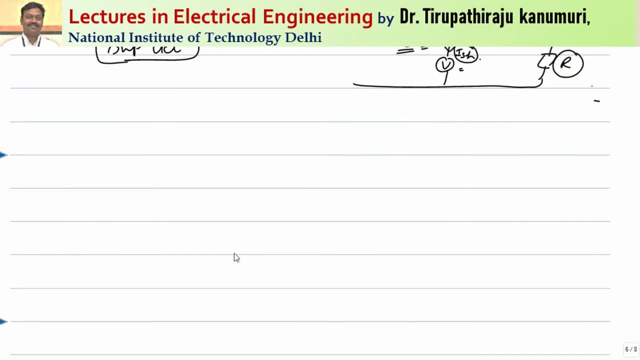 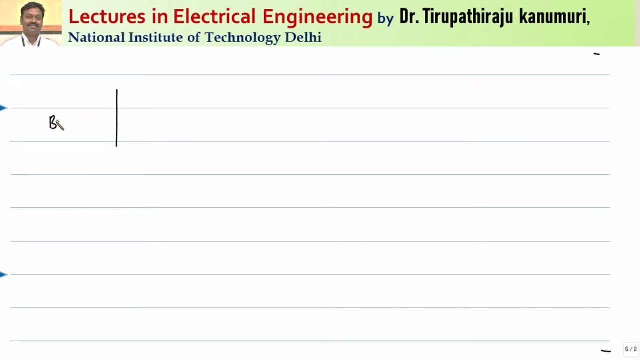 be there so that trip circuit will take the power from a separate source, so that burden will not be there on this ct and the pt and they will operate your circuit breaker either directly or indirectly. so, summarizing this, i am just drawing what are the basic components for the circuit breaker. so 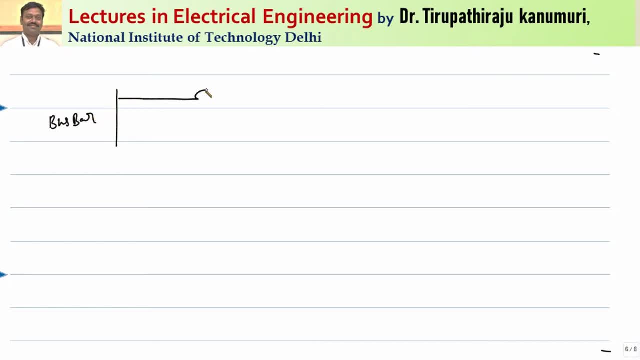 there will be a bus bar. so this from the bus bar, because we have to measure either the voltage or the current. so either ct will be used or pt will be used, or both will be used, depending on your requirement. that is why i am drawing both the things. so these things will be given to. 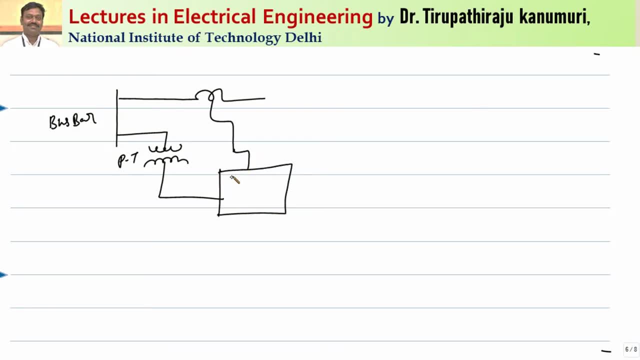 you is a relay, so relay, depending on the requirement, it will use any one of these components. so there will be a relay, so this relay will close its contacts. so the relay will close the contacts of a trip coil or a trip circuit. so this trip circuit will be energized from a battery source. 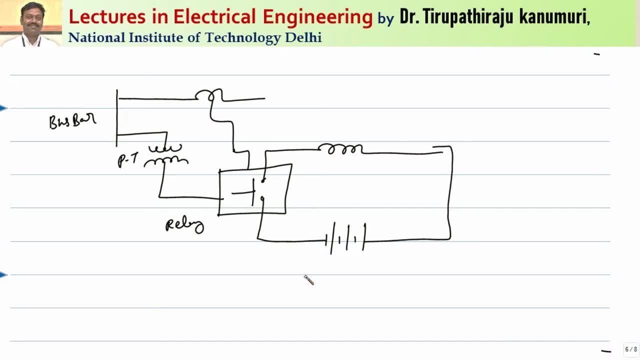 so this will be energized from a battery source. so battery source will be connected to this one. so here there is a battery entire circuit we can call as the trip circuit. so whenever the relay contacts are those, this battery will supply the required for energy for this trip coil. so this trip coil will activate. 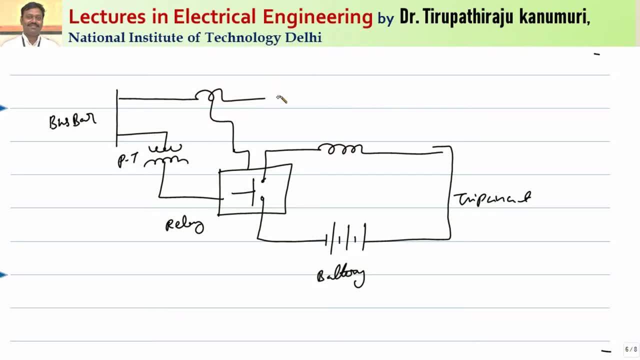 your circuit breaker. so i am just representing the circuit breaker here. so let us assume there is a circuit breaker, so this circuit breaker i am representing by this one. there is a circuit breaker, so this circuit breaker contacts are directly connected to this trip coil. so this trip coil may either directly operate the circuit breaker or sometimes, if more energy is required, 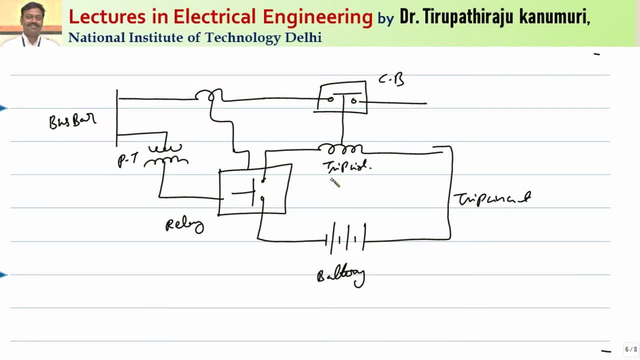 for operating the circuit breaker. so this trip coil may energize the circuit breaker opening circuit, so the circuit breaker opening circuit can operate it, or directly, if the energy required is this directly, the trip coil can directly operate the circuit breakers. so these things we are going to see in detail when you come to this respective topics. so let us see each one of. 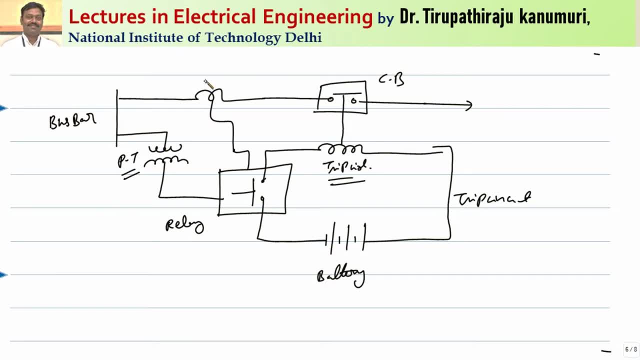 these topics. so first thing is coming to the ct and the pt generally, this current transformer and the potential transformer for the case of protection purpose. generally they operate under the fault conditions. that means during fault conditions the voltages or currents will be abnormal: either they will be extremely high or extremely low. so 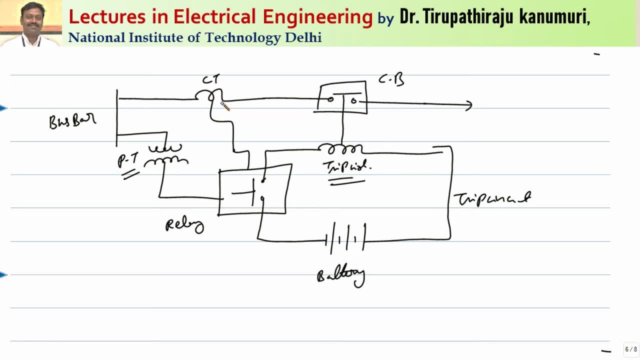 the magnetic characteristic of this or the bh characteristic of these. both these circuits should have the linear characteristics and they should not get saturated so that the effective outline and theIlupi voltage, if this is, if it is allezness here- any current comida too high. 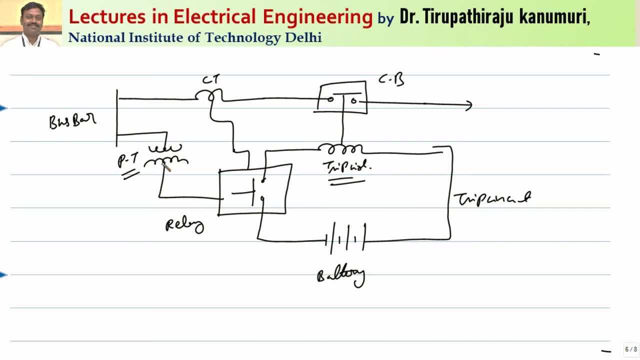 over time for this and this VPN you can see posted here. but in the case of Cchoolyrics actually popped around this. there are also部分 dass anyd capacitor cloth. it should not pry out the relay. there should be no. well, as a split relay comes- asked that is in the previous video- say product voltage, the star period. 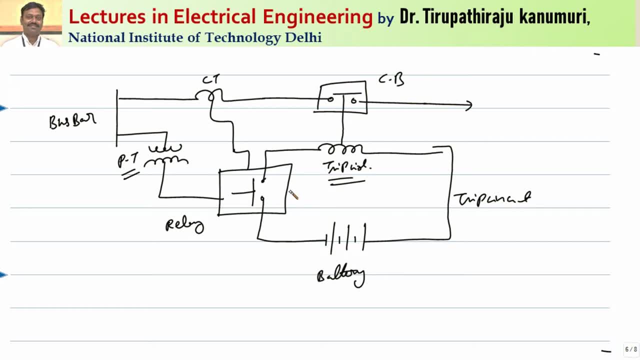 of A thing. it also cantez also can z Sang off the right. so this case we fix the current relays, earth fault or zero sequence relays. different type of relays are there. so those things we are going to discuss in detail in the module number three. so after that, once the relay 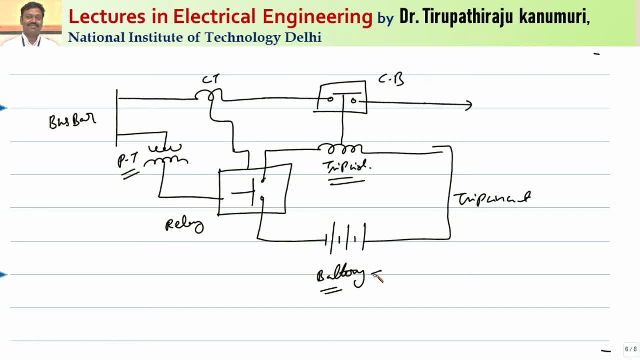 is closed. it will close the battery circuit, so this battery should have the sufficient energy to activate this tripping coil generally. what will happen practically? practically, instead of using a battery, let us assume i am directly stepping down the voltage from your supply. that means i connect a transformer from your supply and activate this trip coil. but whenever the fault, 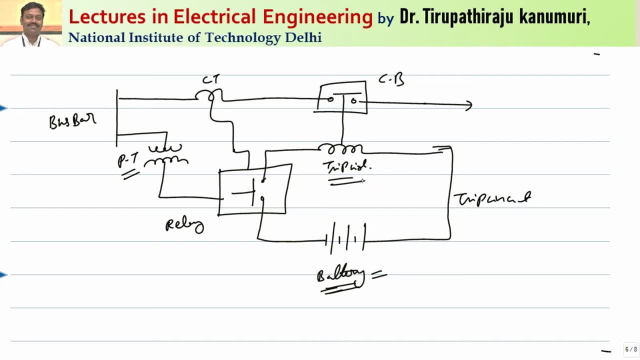 comes, we know the voltage will drop to zero or to a very less value. when the voltage drops to a less value, that cannot supply the required power for this trip coil. and sometimes let us assume the substation where this trip coil is there, that substation itself is disconnected and sometimes 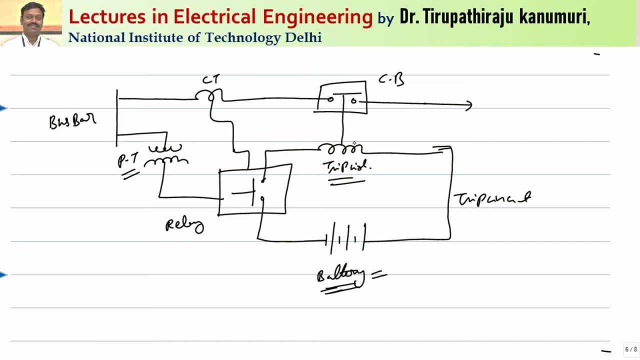 it may take some eight to ten hours to completely rectify the fault, so for that much time the battery should be able to supply this. that's why a separate battery power bank is provided at each substation, and this battery power banks takes the power from the supply only. it will charge it and whenever the power is not there, in your 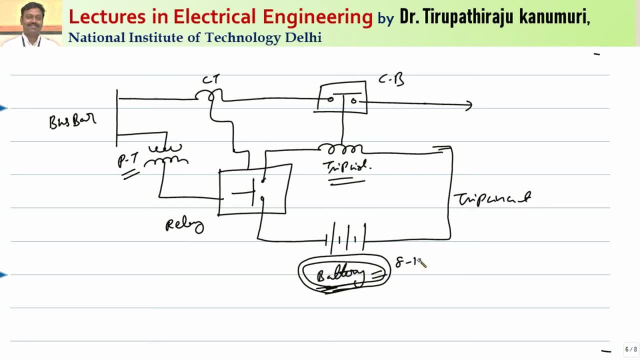 substation that can supply the required power for up to 8 to 12 hours of time. so this much sufficient capacity should be there in the battery circuit. now coming to this trip coil. so the trip coil will activate a circuit breaker and circuit breaker will open. so now coming to 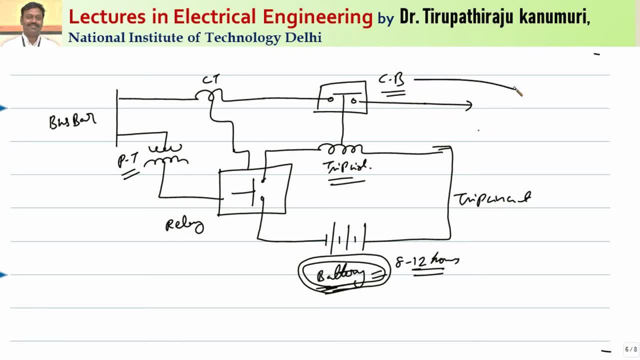 the circuit breaker. so circuit breaker will have two things. so, coming to this circuit breaker, the circuit breaker will have the two contacts. one is the fixed contact and the second one is moving contact. so one is the fixed contact, second one will be moving contact. so now the moving. 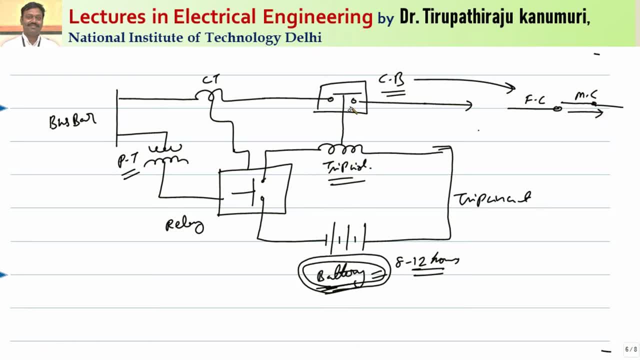 contact will move. whenever the fault actuated, that means the trip coil actuates, the circuit breaker, the moving contact will move. so whenever the moving contact is moved, so there is a fixed contact. let us assume moving contact has moved up to here, so moving contact is moving like this, so automatically. 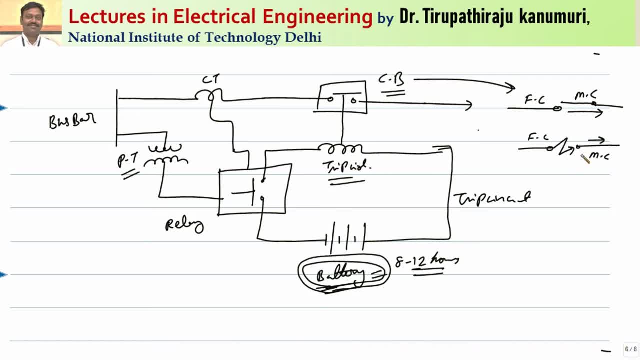 the arc will struck up between these two contacts and the trip coil will actuate the circuit breaker and this arc creates the huge value of the heat. because of the heat the contacts may spoil and generally what happens. because your supply is sinusoidal, some point will come where your current 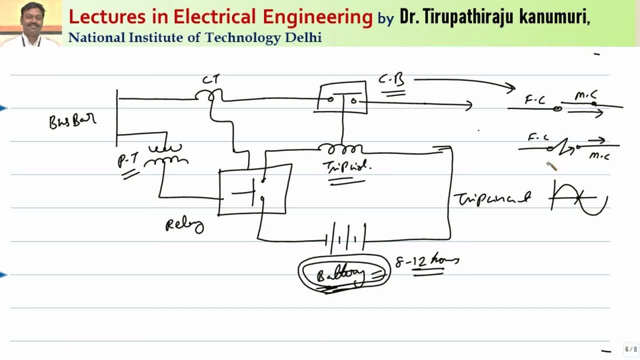 will reach zero during the current zero because there is a arc, because in between there is a vacuum, or the gap will be there or some intermediate medium is there. so the arc will get extinguished at current zero, but whenever the arc get extinguished, so there is a concept called as a 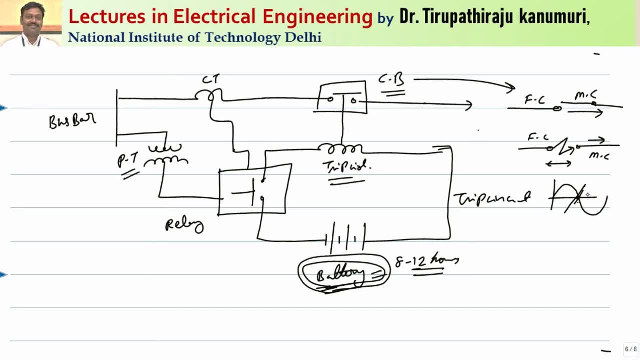 restriking voltage which happens due to the inductance and capacitance of your system or the energy storage elements, and that restriking voltage may be sufficient to restrike the arc again. so a proper medium should be provided which will not allow the restriking of the voltage because which? because of the effect. 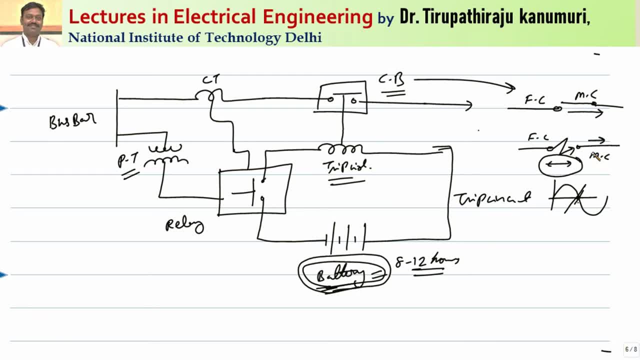 of the restriking voltage, the voltages may increase to a drastically high values and that may spoil your equipments. so these things we have already seen in the case of traveling waves in power systems, so you can please refer there if you have a doubt about these things. 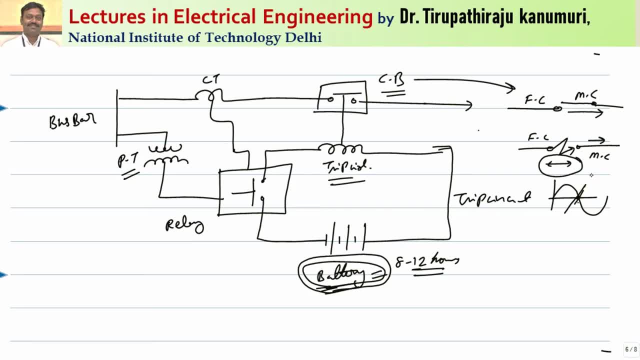 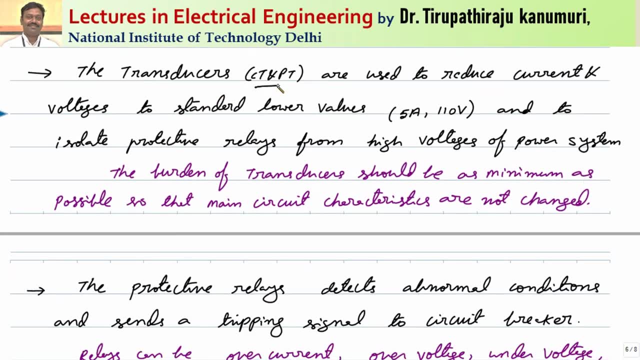 and remaining details we are going to see in the case of circuit breakers. so now i am going to summarize what we have seen till now. so first is the transfusers you are taking, ct or pt, are used to reduce the current and voltages. so a standard, lower values. generally, standards used are 5. 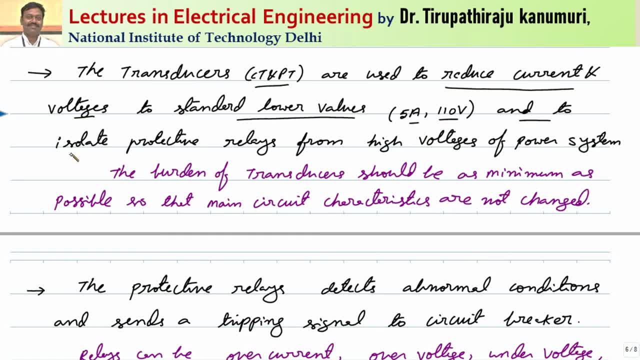 amperes and 110 volts and to isolate the protective relays from high voltage of power system. so you may have doubt some book i have read. this is not 110 volts, it is less, or they have mentioned 1 ampere. actually i am telling the standard things that are used for 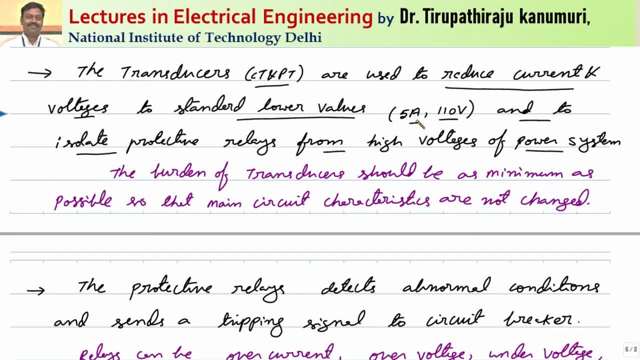 electromagnetic relays. if you are going for the static relays, because this much current and voltage is also not required, it may be lesser values than this, but generally the standard values that are used are 5 amperes and 110 volts only, so the burden of transducers should be as minimum as 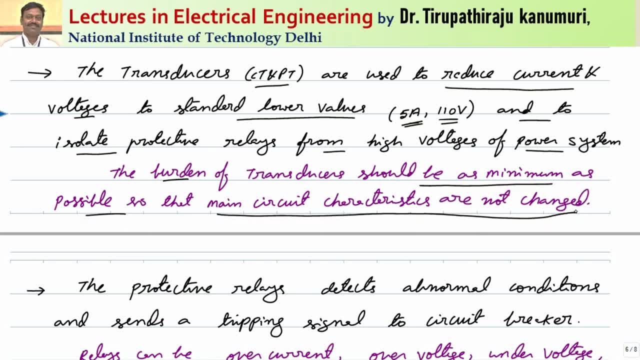 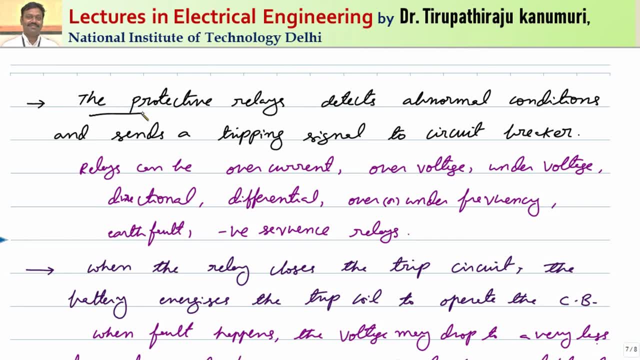 possible so that the main circuit characteristics are not changed. i have told you the reason: because otherwise they will affect your main circuit characteristics, so that should not be. then the protective relays detect the abnormal conditions and sends the tripping signal to the circuit breakers. so these relays can be either over current type, over voltage, under voltage. 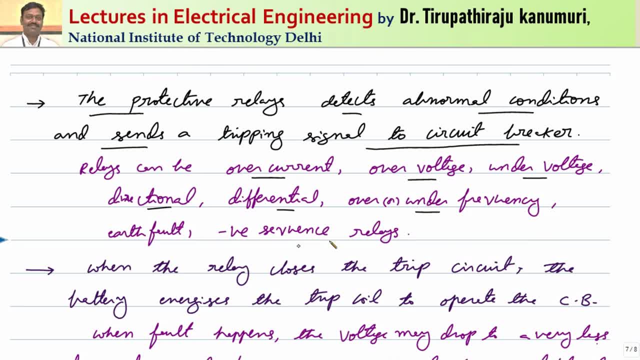 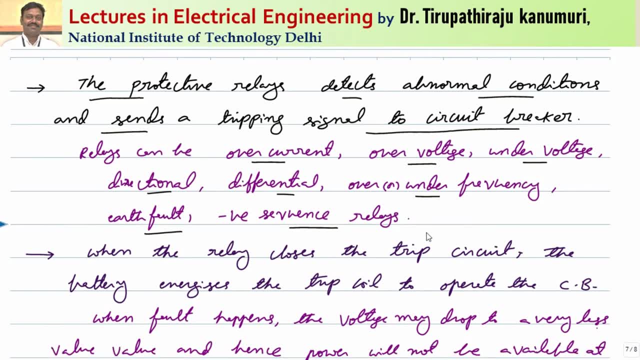 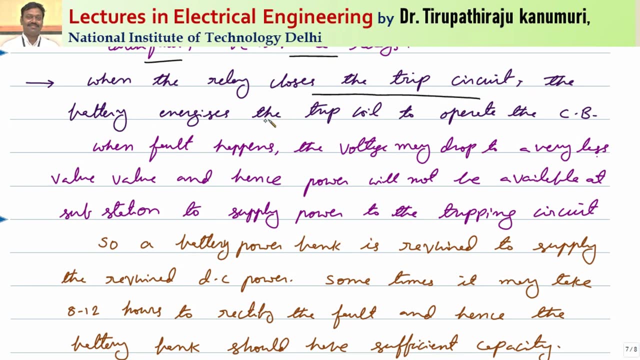 directional, differential, over or under frequency, earth fault, negative sequence, to name a few type of the faults. there are some more other type of false relays also that we are going to discuss in detail in the next module. so now, when the relay closes the trip circuit, the battery energizes the trip coil to operate the circuit breaker. so so generally, what happens? 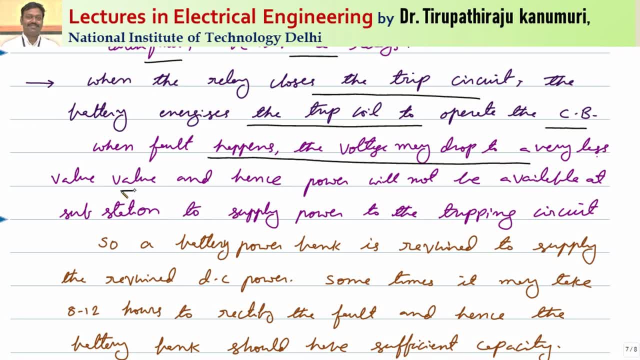 when the fault happens- i have discussed this- the voltage drops to a very less value and hence power will not be available at the substation to supply the power to the tripping circuit. so what should we do? a separate power bank should be required to supply the required dc power. so sometimes 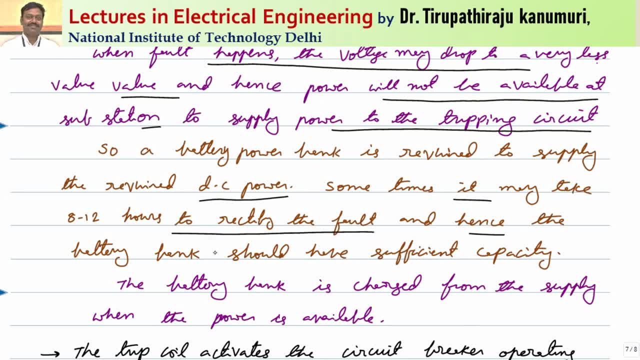 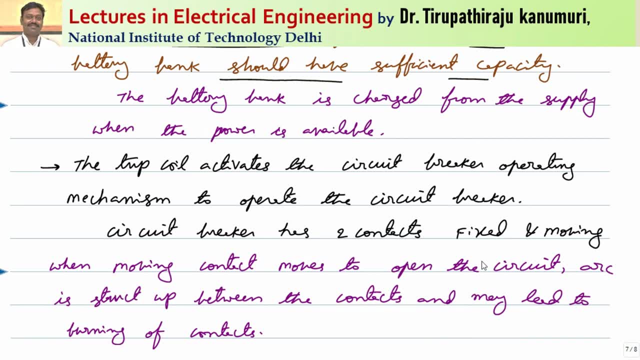 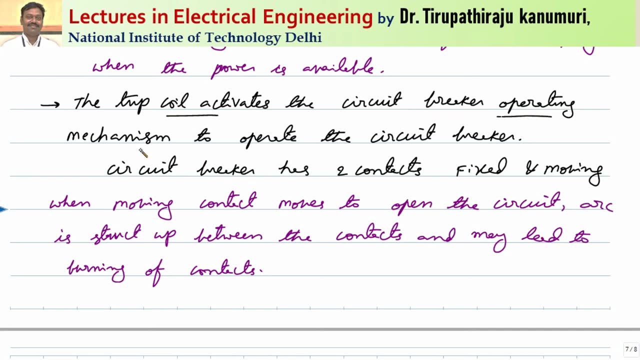 it may take 8 to 12 hours to rectify the fault, and hence the battery bank should have sufficient voltage to supply this power. so the battery bank is generally charged from the supply only when the supply is available. now coming to this trip coil, activate the circuit breaker operating mechanism.